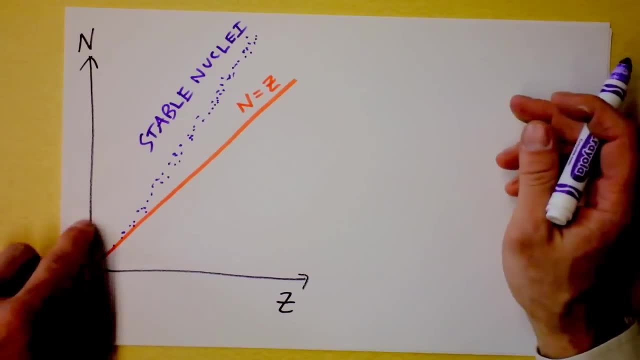 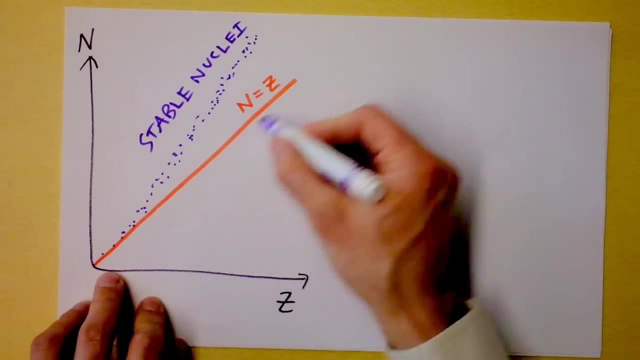 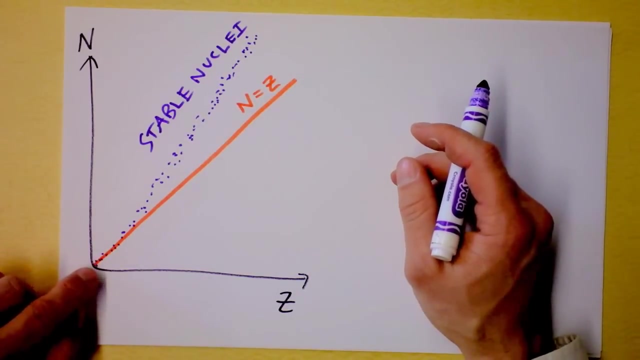 And this: this graph is a graph of the number of neutrons versus the number of protons in an atom, And I've graphed the line n equals z because early on these data points the stable nuclei do follow the general pattern where, if you've got another proton, 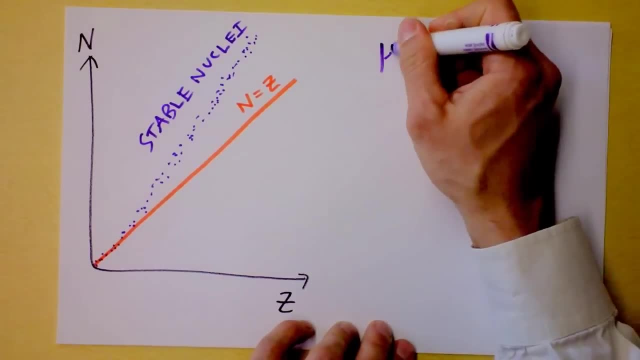 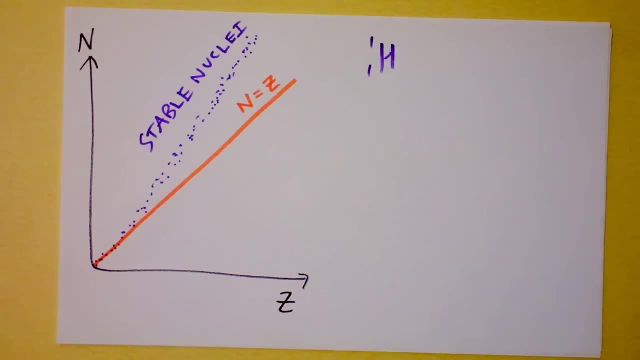 you're probably going to need another neutron. So let's just look at some examples. If you look at hydrogen, you can have hydrogen where there's there's one proton, right And one- oh, I mean no neutrons. You can also have hydrogen where there's two. well, there's one. 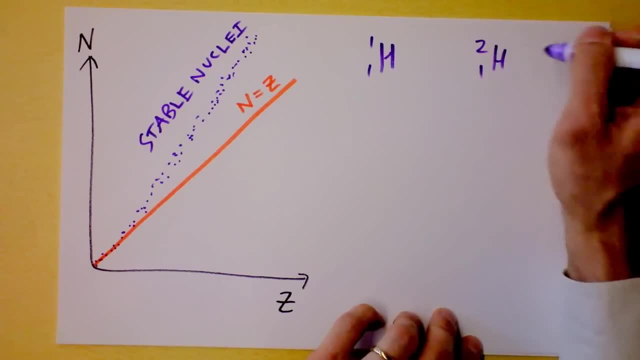 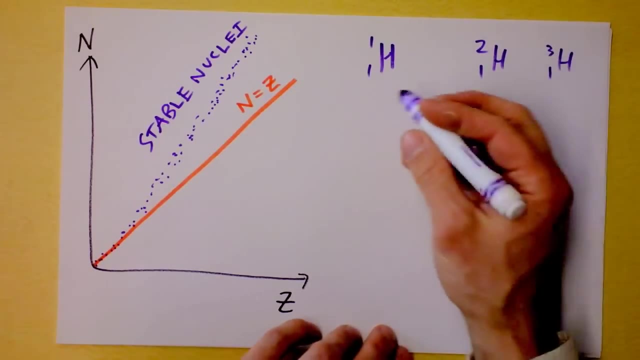 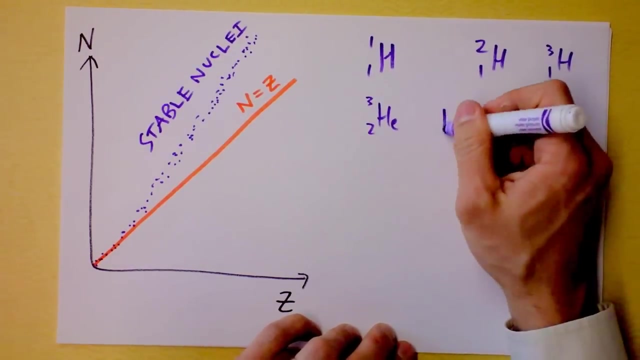 neutron and one proton, because then this is A right, And then so that's called deuterium. You can even have tritium. This is not stable, though. That's the problem. Deuterium will last you for a long, long, long, long time, But then you can have helium, and you can have helium three, or you can. 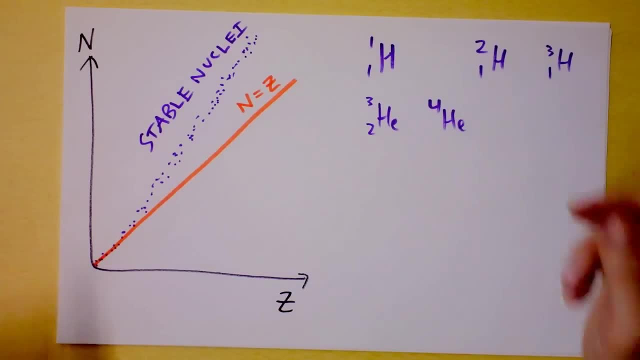 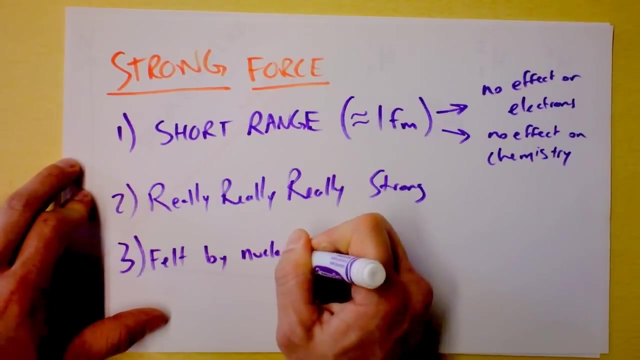 have helium four. It prefers to be in the helium four form, though, because you got two protons and you've got two neutrons, So neutrons must feel this strong force Felt by nucleons. So it's felt by protons and neutrons. So the nice thing about neutrons is they. don't add anything to the repulsion force of the nucleus, which is just from the protons, but the neutrons do contribute to the glue that is gluing these nuclei together. So it turns out that as you get even heavier, bigger and bigger atoms, you need to have disproportionately more. 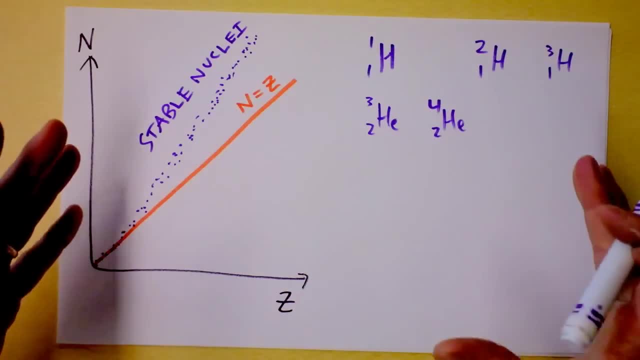 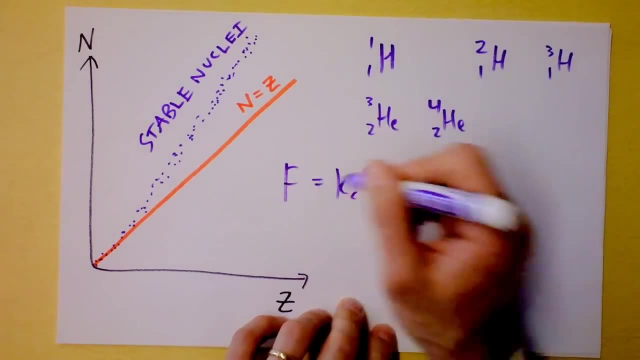 neutrons because you need to space out your neutrons. So you need to have more neutrons and you need to space out your protons a little bit more, because the electrostatic force of course KCQ1Q2 over R squared, depends heavily on distance And as you get these guys spaced further apart. 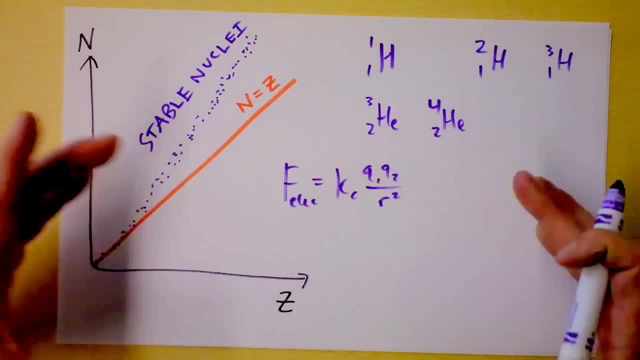 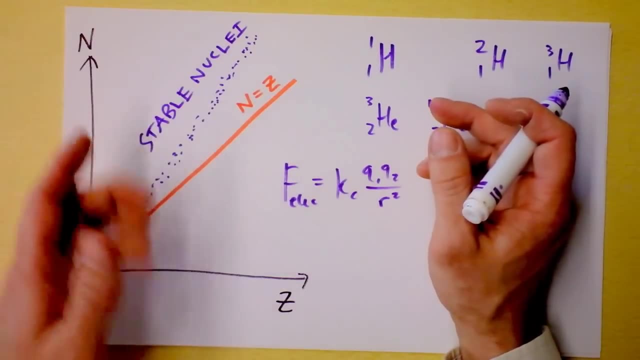 with more neutrons. you don't add to the force, You merely diminish the force, but you've still got this strong force happening here. So here's a question for you: Why not have atoms that have enormous number of neutrons and very, very few protons? Why aren't there more stable things over? 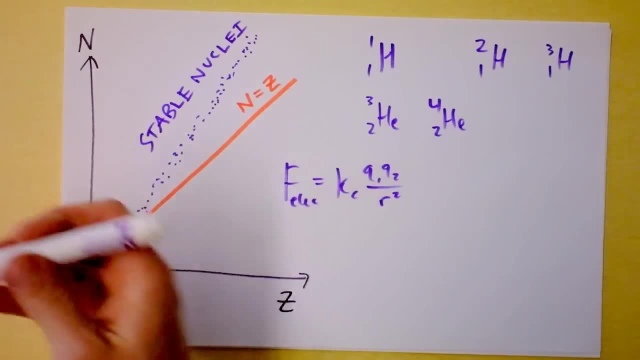 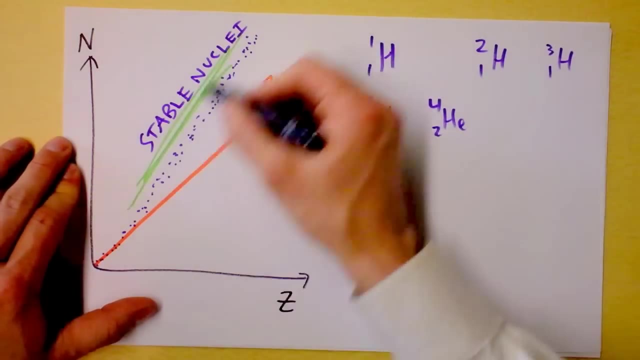 here And we'll talk about why that's the case. Turns out, just a few of them are stable, And if they're not stable, then they're going to be decaying in various ways. So I'll draw some lines over here, Generally the ones that are on this side of the 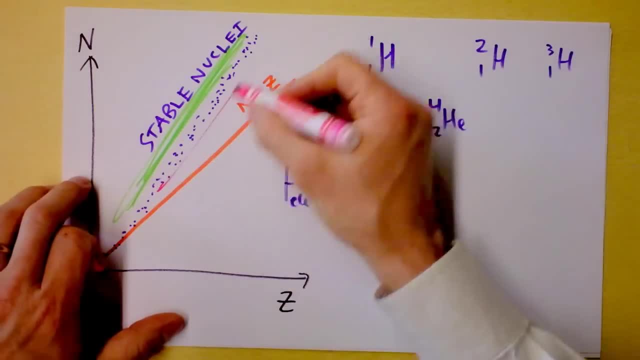 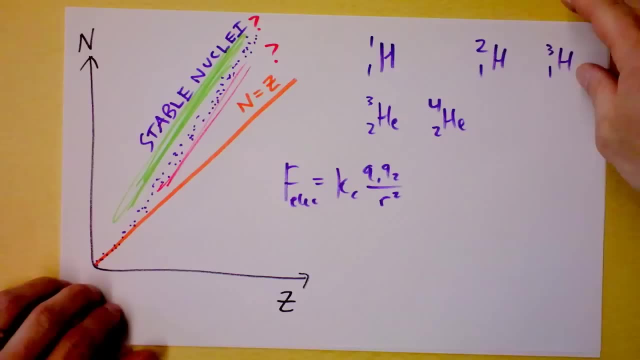 graph are going to be decaying in one way And the ones that are on this side of the graph are going to be decaying in another way, And these decay modes are things that we'll talk about in a little bit, But let me introduce you to a little bit of radioactivity. Becquerel discovered radioactivity. 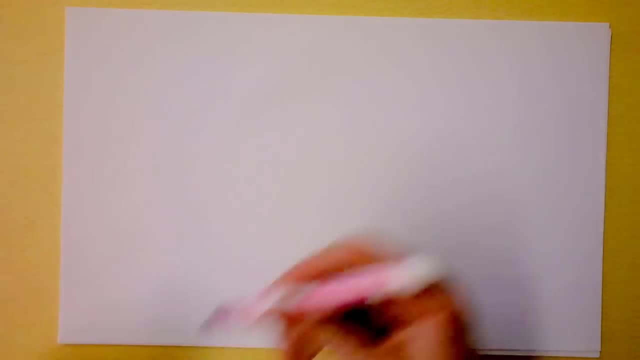 It's really a French thing. And then Madame Curie and Pierre Curie were all about radioactivity And shortly after 1900 happened 1905, there was a ton of experimentation that was happening on radioactivity. So one of the cool things about radioactivity is that if you put a radioactive 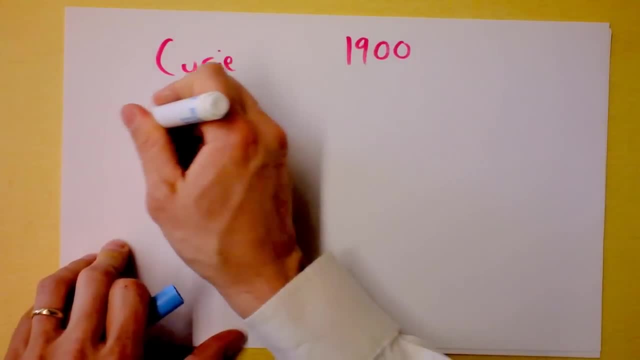 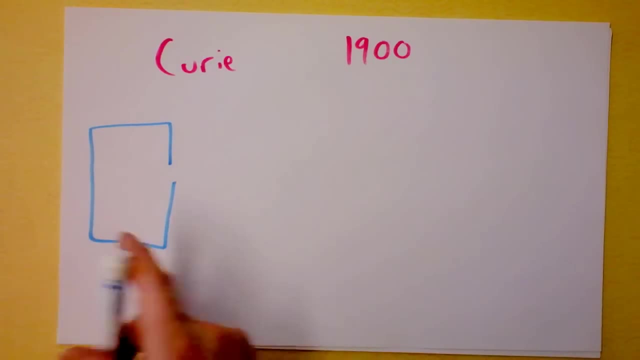 thing in a box right here. you find that there are rays coming out of it And they called them alpha, beta and gamma rays, And I want to talk to you about these three different types of rays. I'm setting them in a box And here's my radioactive stuff. 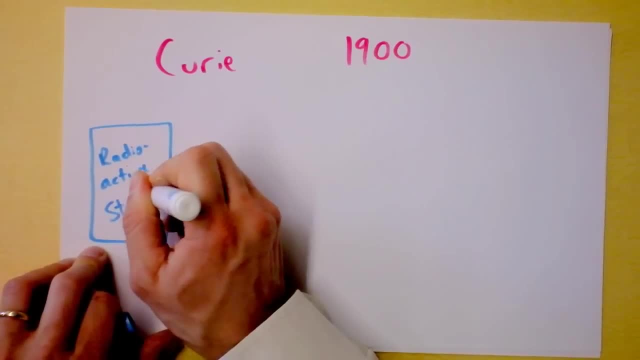 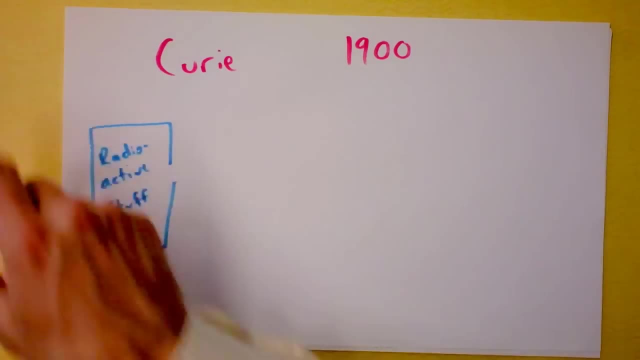 Radioactive stuff. I don't even care what it is- Uranium, plutonium, americium, whatever you want to put in there- But we put this in a box And then outside of it I'm going to make a magnetic field And I'm going to have that magnetic field pointing in all the 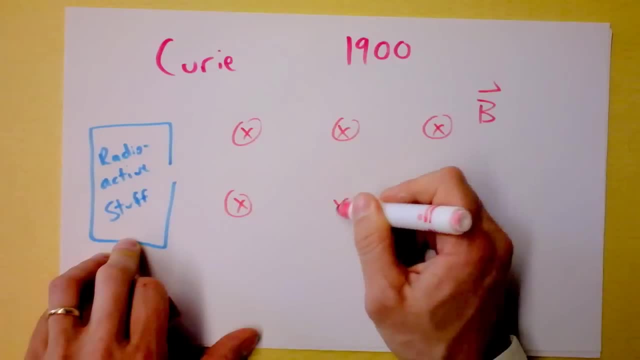 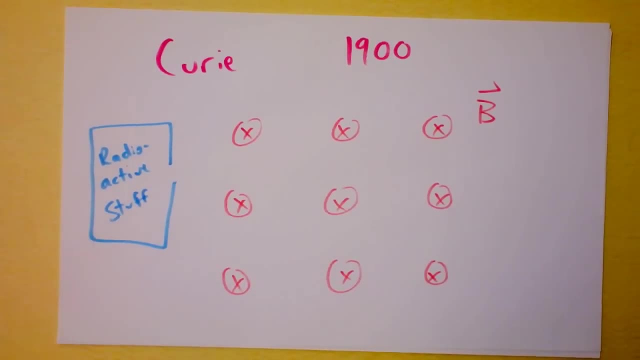 time. Here's my magnetic field B, pointing in all the time. And they did this and learned that there are generally three paths that the radioactive stuff will form. Some of the radioactive stuff just went straight out of the box And they did this and learned that there are generally three. 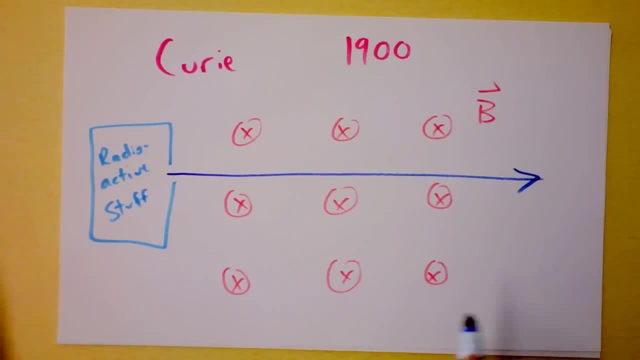 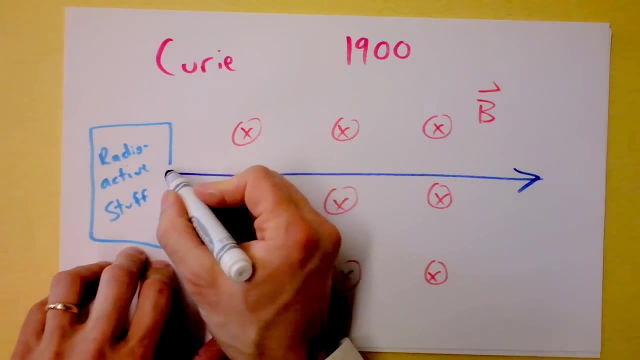 paths that the radioactive stuff will form. Some of the radioactive stuff just went straight out of the box. Pew Right, Some of the radioactive stuff generally, some of the radioactive stuff, decided to go like this. Let me see if I can get this right. Yeah, Oh yeah, It went like this. It went just slightly. 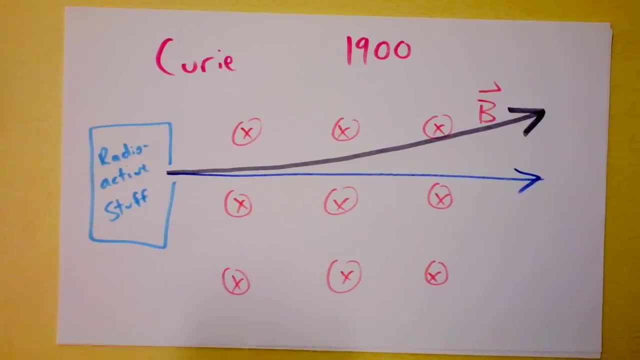 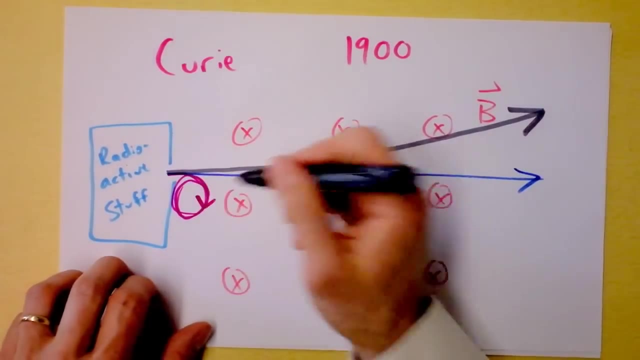 curving that direction. And finally there was a type of radioactive stuff that came out of here and went pew And went around a little circle here, right, Wow, That's really curvy compared to those guys that are just a little bit curvy, Interesting. 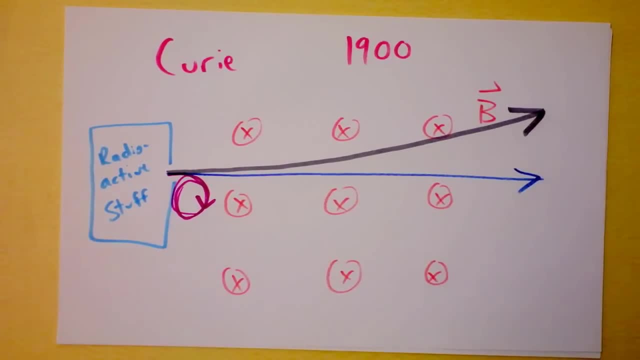 All right, Let's look at what they named these guys. They called this one alpha, And they called this one beta And they called this one gamma. Turns out that those are the first three letters of the Greek alphabet, So they just wanted to label these three types of radiation: alpha, beta. 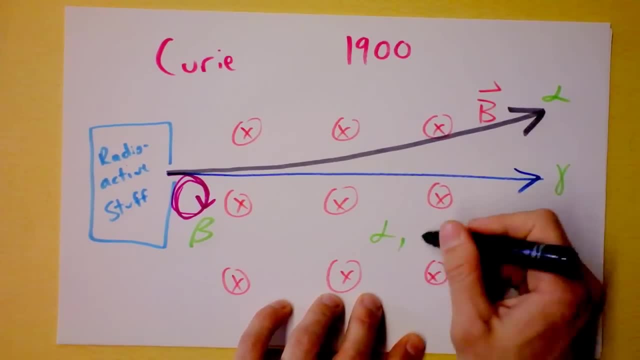 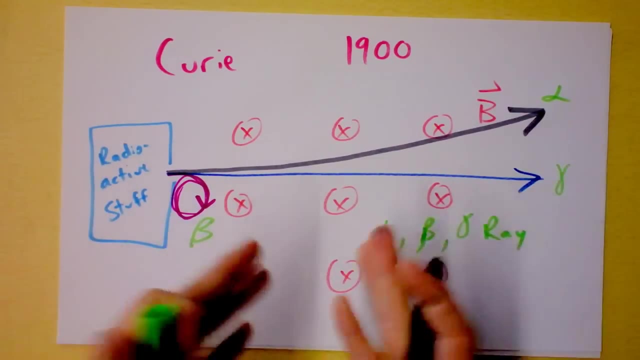 and gamma rays. So you got alpha and beta and gamma rays, And that's radiation. They are radiating, They're coming out in straight lines, unless there's a magnetic field on, in which case you can get them to separate and learn more about them. So I'm going to distinguish these three types of rays. 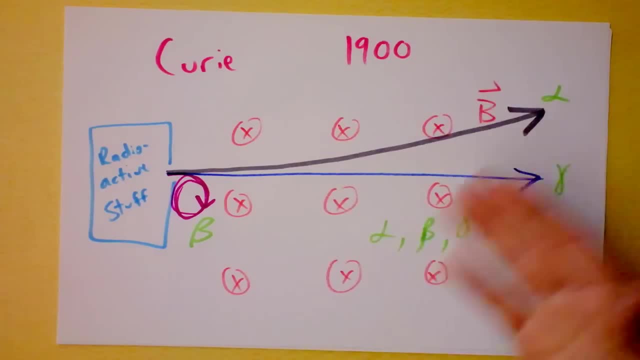 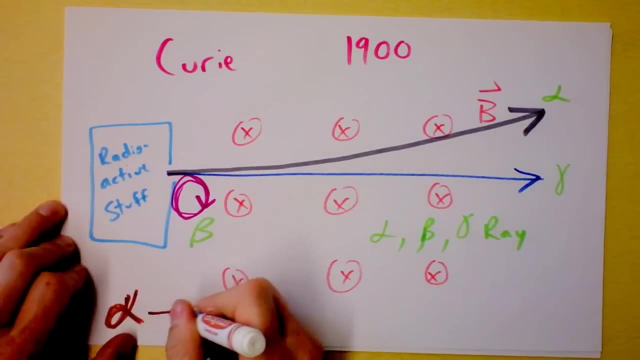 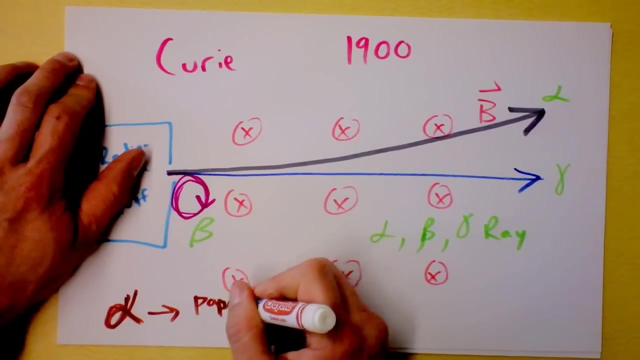 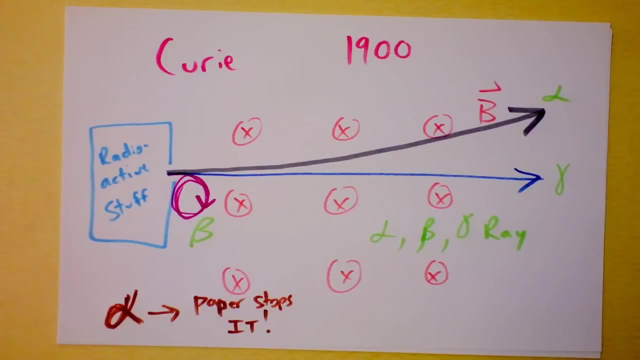 The names are stupid nowadays, but they stuck because of this original sorting procedure: An alpha ray. Now it's known that an alpha ray is actually particles. An alpha ray does not penetrate very much. Paper can stop it, Wow. An alpha ray, therefore, is not particularly dangerous As long as you're behind a sheet of paper. 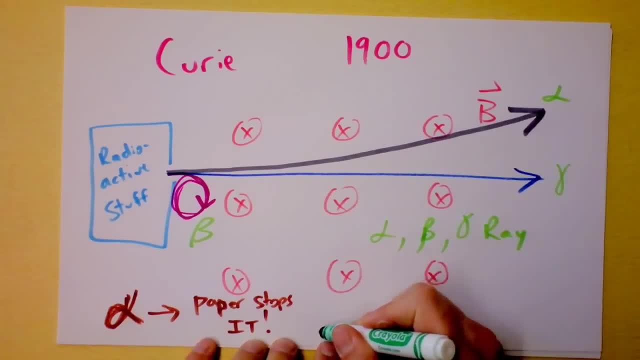 for your defense. an alpha ray can't really hurt you. What about a beta ray? The cool thing about beta rays is they are a little bit more dangerous. You need to get aluminum foil to stop it. Uh-huh, That's a little bit scarier. You wouldn't want to let beta rays hit your skin. And then what? 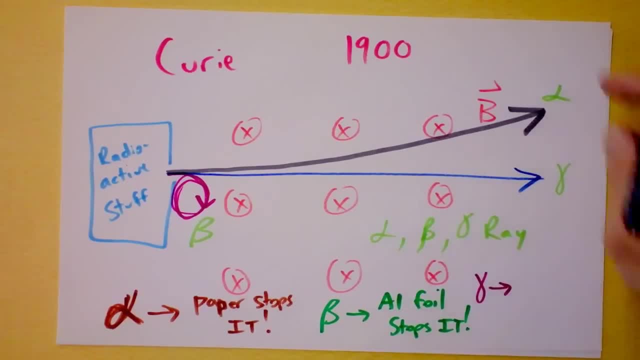 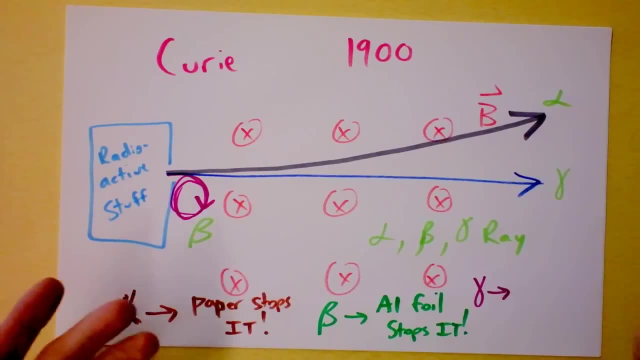 about this guy called the gamma ray. Gamma rays are a major problem. Gamma rays can go through several centimeters of solid lead. That's an enormous amount of mass And this ray just shoots right through it. Let's see Several centimeters of lead. I'm going to have to talk over that guy, so I think I can do it. 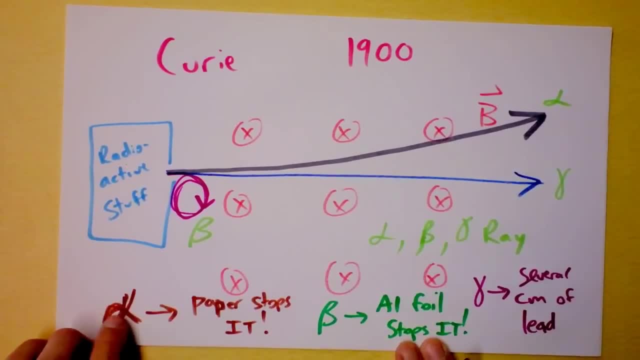 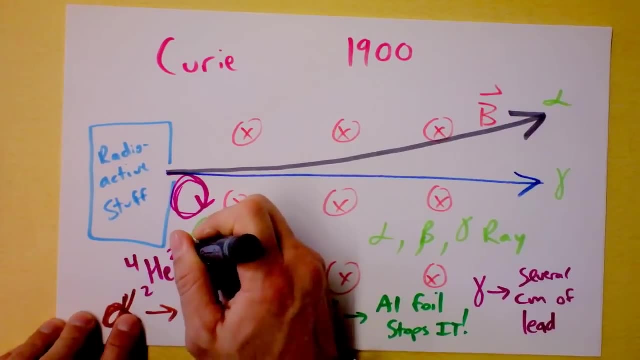 All right. Several centimeters of lead. aluminum foil stops beta rays. These guys right here are helium nuclei. Helium nuclei, We're talking about 2,, 4, and I'm going to have a 2 plus right there because it is very positively charged. 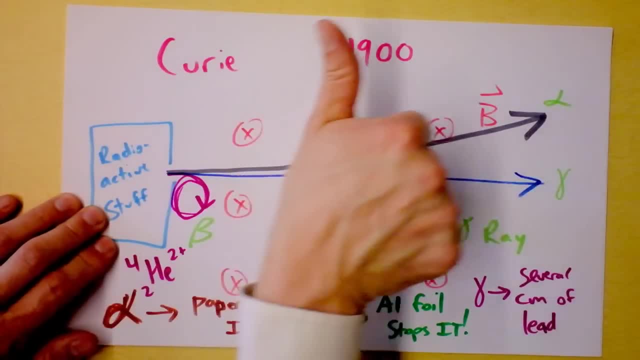 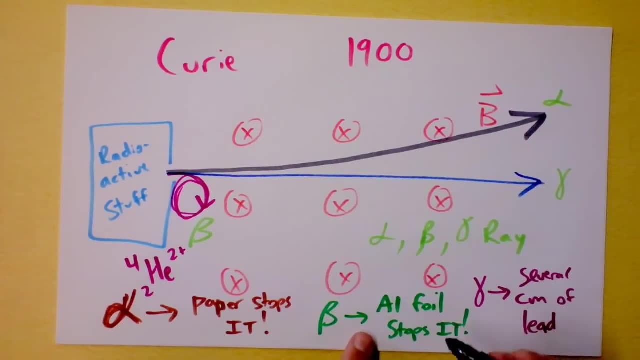 Notice that if I have my velocity, that direction the magnetic field's in. then the force will be upward on it, But it's got a lot of mass so it's not going to turn very much. Ooh, beta rays. I'll tell you about beta rays right now. 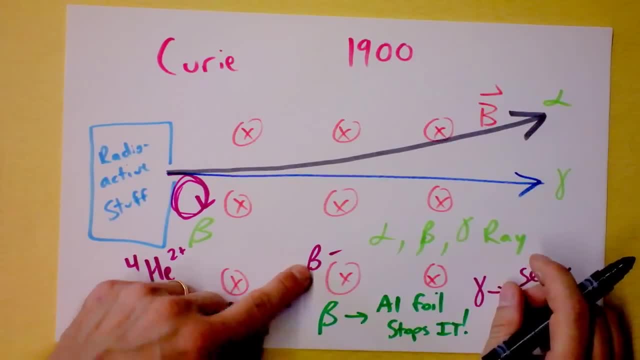 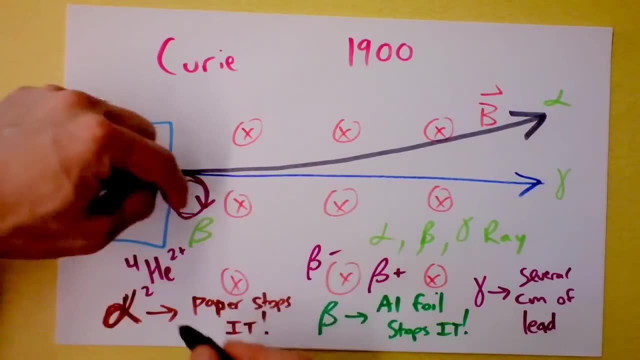 Beta rays are just electrons and a lot of people call them beta minuses, because there's another thing that's called a beta plus, And this is the opposite of electron. It's a positron, Alright, so that guy will turn like that because it's negative. so I have velocity coming that direction.